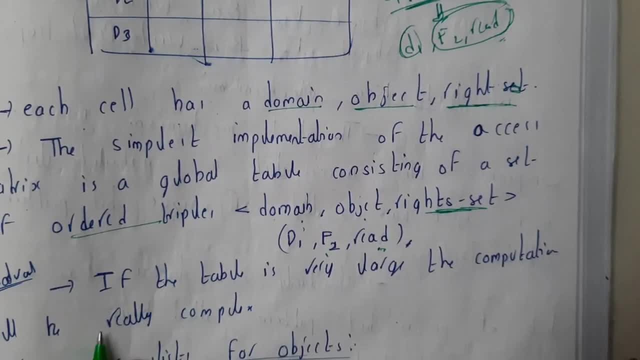 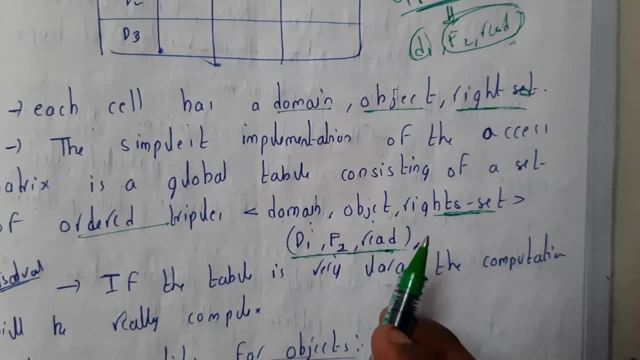 way. So the basic disadvantage of it is, if the table is really large, then computation of each and every cell will, in this format will be really complex, because it is a hectic work to do. So that's the reason why this global table is not similar. All right, So. 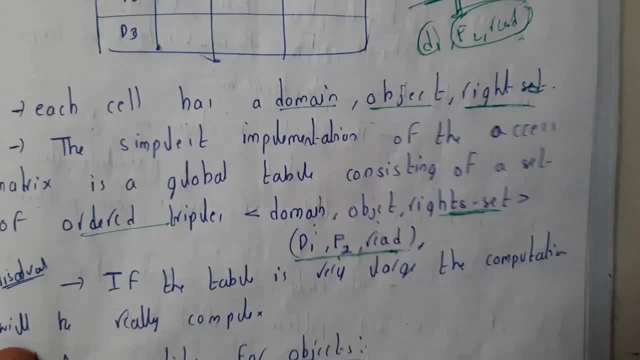 we're going to try one more time. Okay, So now we're going to try one more time. So this is the basic disadvantage of it is, if the table is really large, then computation of each and used so after that. the another way of implementation is access list for. 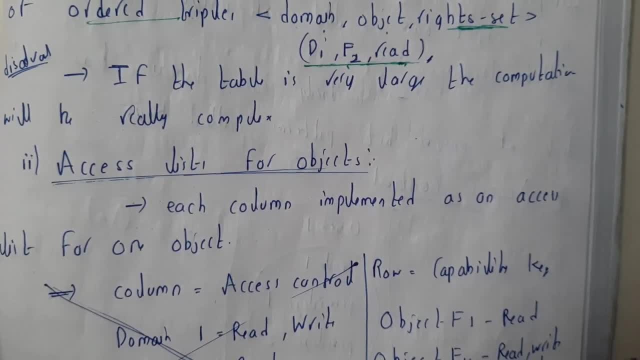 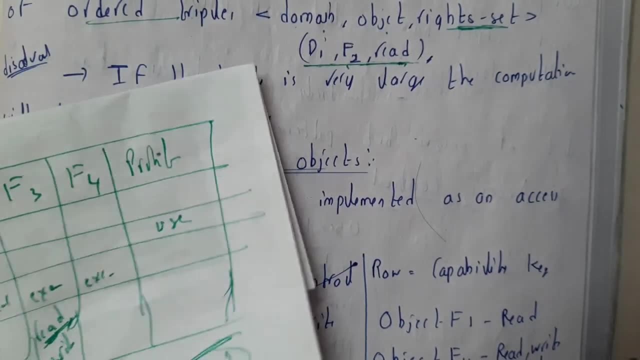 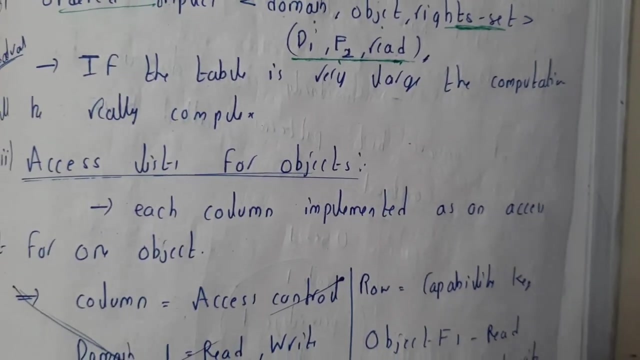 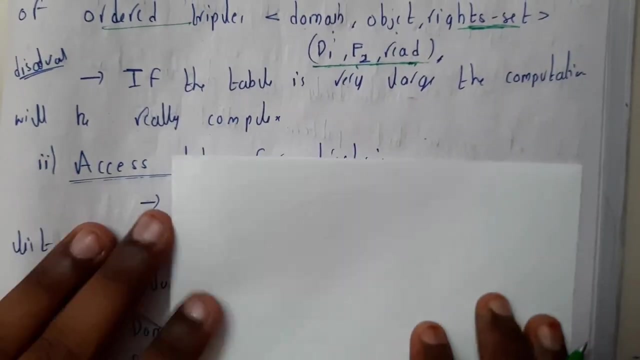 objects for. so we'll be considering only access for object, guys. so, basically, if you take a small example, so let us take the previous example. is it clear, or shall I write it again? I'll be writing a different example. just give me a second. I'll be taking a piece of paper. just a second, guys. okay, so I took a small piece. 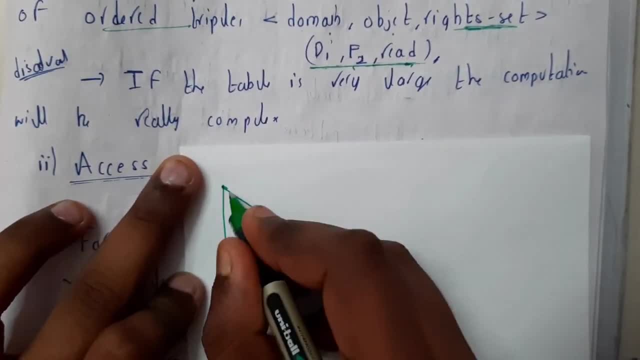 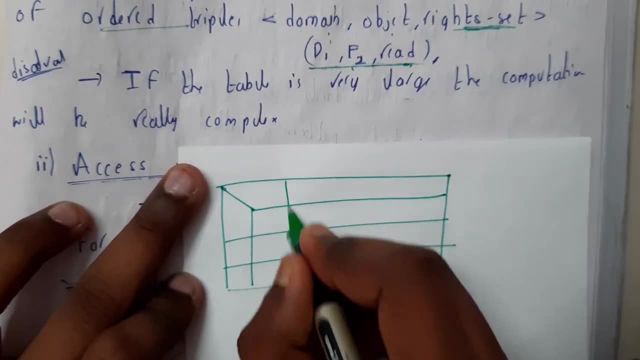 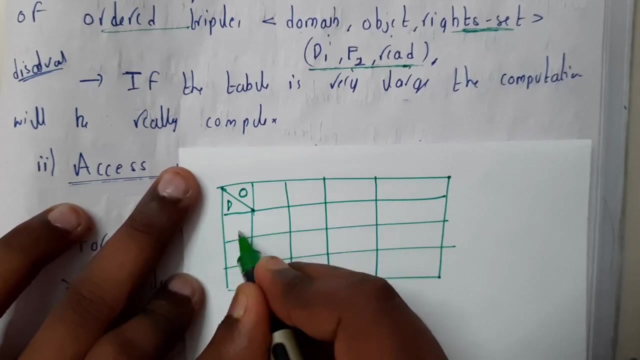 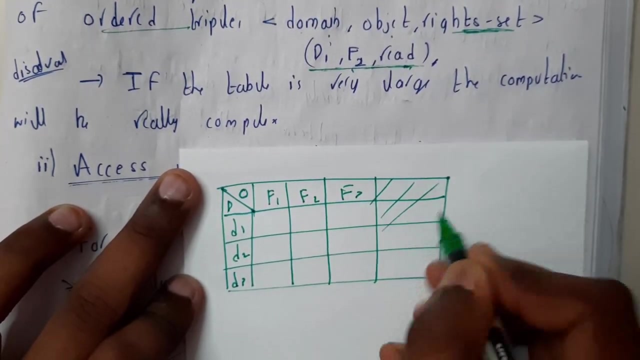 of paper, so let us write for three, it will be better. four, I gotta be fine, it's okay. so it is nothing but object. this is nothing but domain d1, d2, d3, you have fun. f2, f3- assume that it is not there. fine, okay, so here I'll be writing. 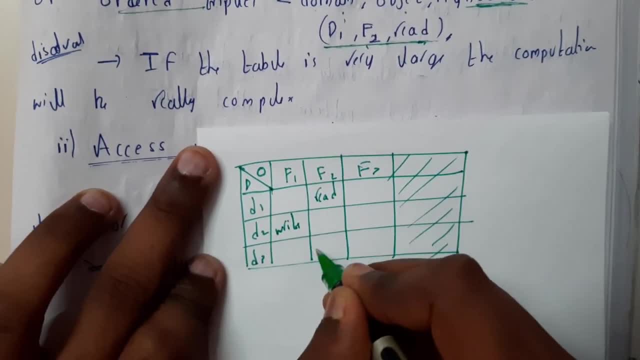 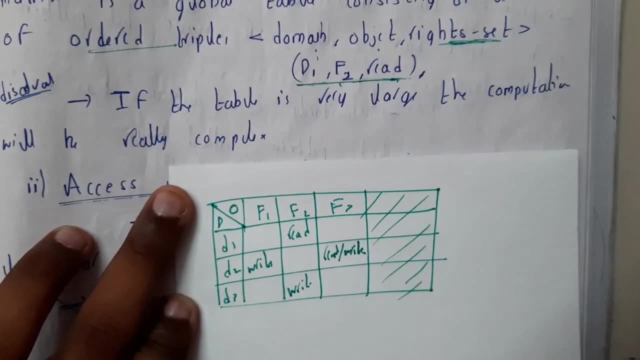 read here. I'll be writing right here. I'll be writing right here. I'll be writing: read or right. fine, I think it's clear. now it's a bit clear when we can come back to the previous one. okay, so now your question will be: what is this? 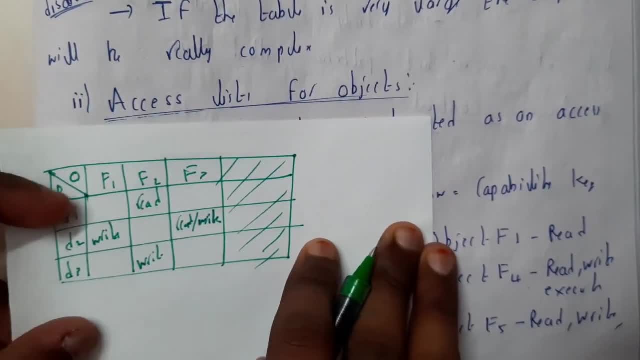 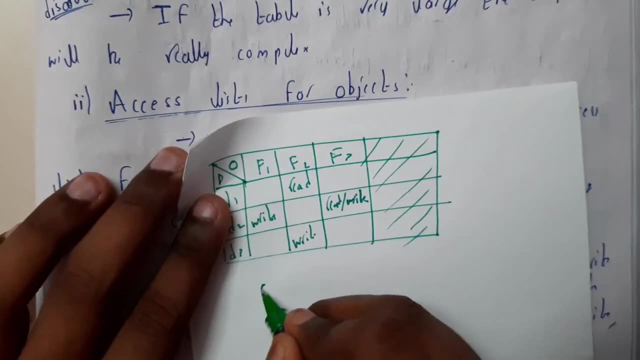 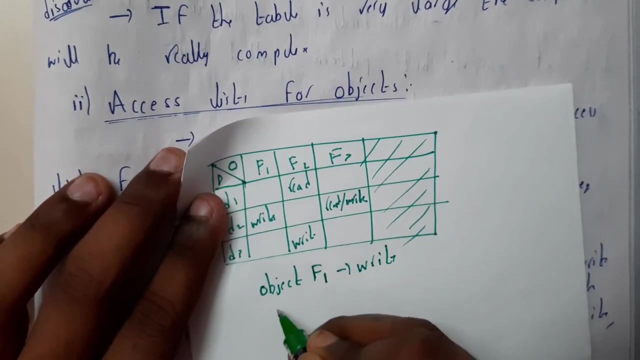 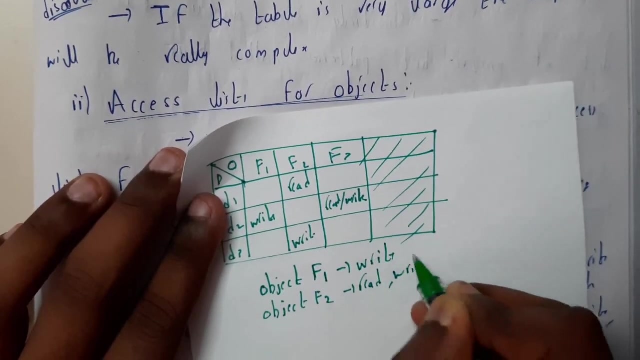 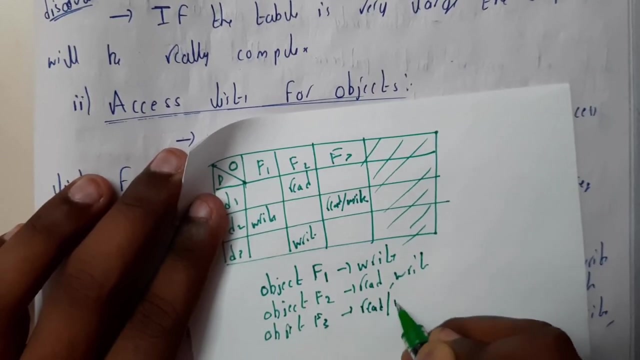 access list object. so basically access list object is nothing, but you will be writing the access rights for this object, guys. so basically we are having object of 1, so object f1 can only write, whereas object f2 can read, comma write where object f3 can read or write. so this is the result that we will be using to 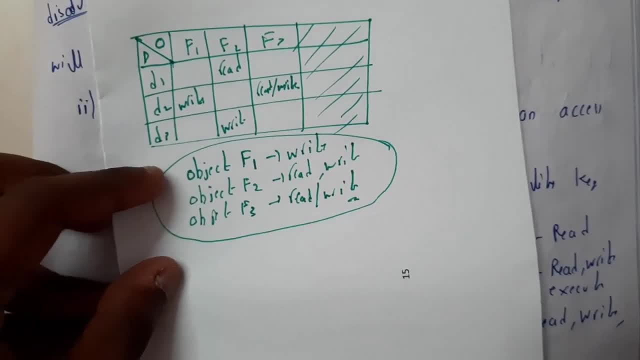 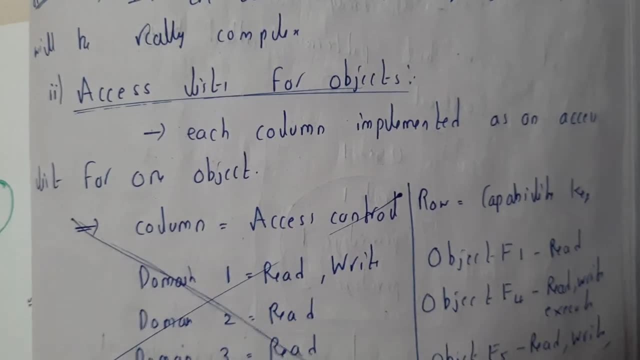 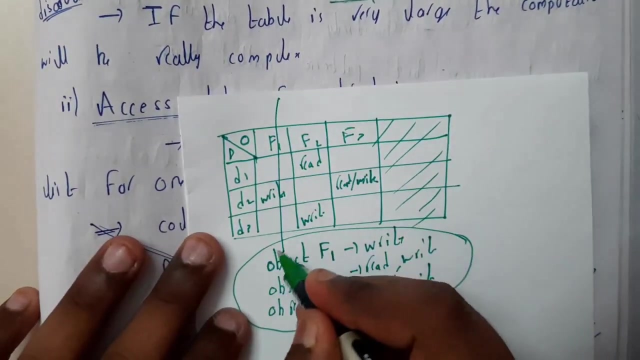 compute it really faster if we store in this way, guys, it is really easy to easy. right, it is easy, but when there are many, many, many large and large tables, it could be a bit complex. so here each column. so what is this, guys? this is nothing but a column, right? so each column implements as an access list. 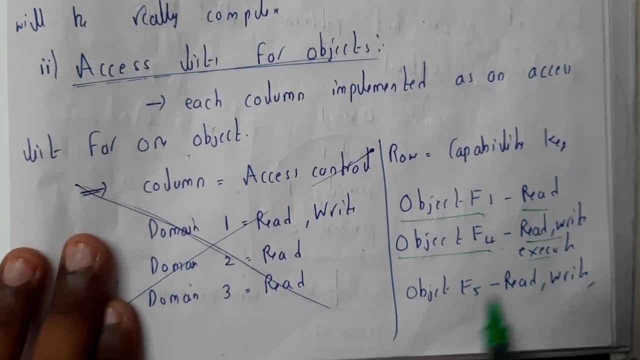 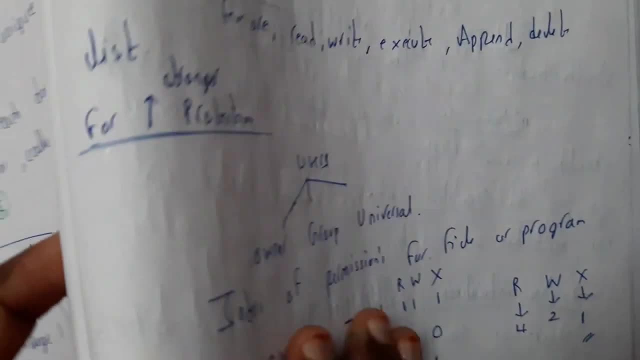 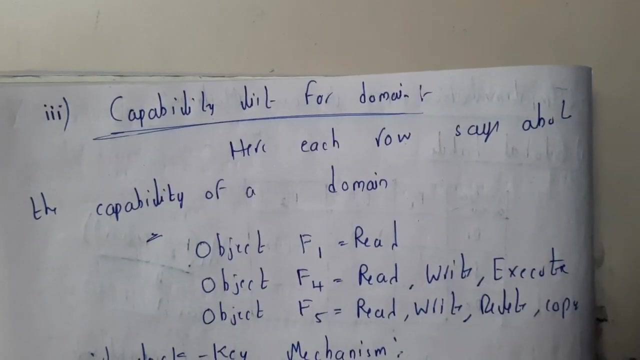 object. so object F1 equal to read. object F4 equal to read, write, execute. object F5, equal to read, write. so this is a basic example without table. I have just took a random example. yes, fine, so similarly we are having for domains also, it is called as capability list of domains. so in this we will be 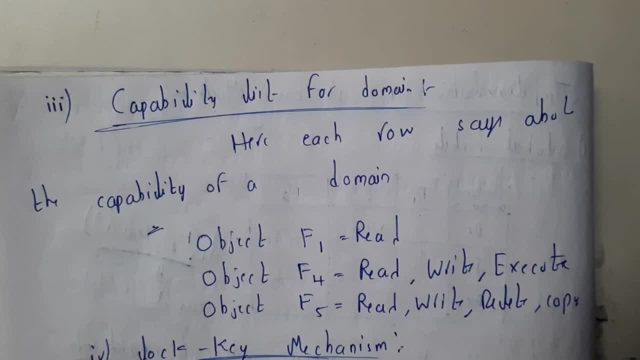 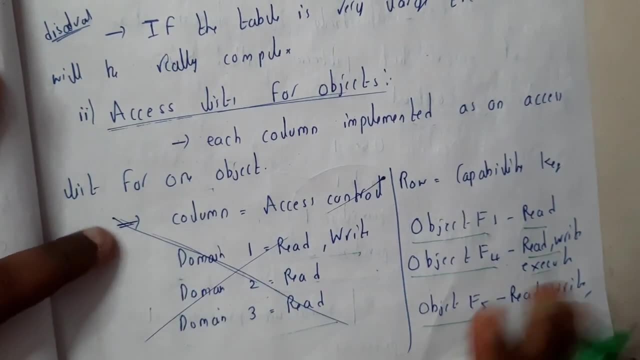 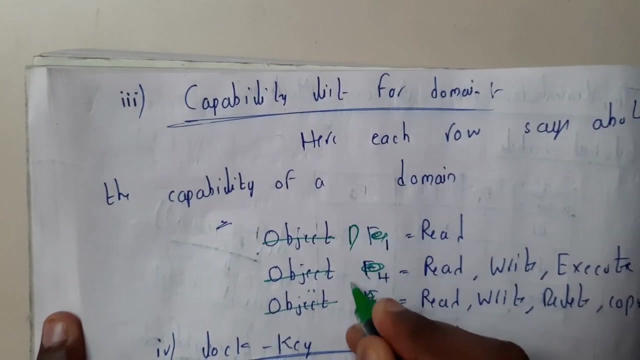 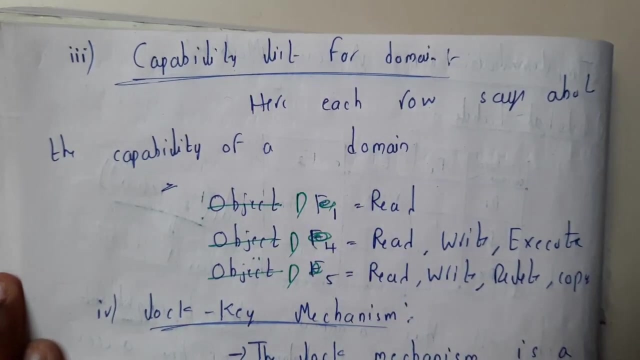 considering the domains. okay. okay, I think I did a mistake here. this should not be written here. this should be written. domains before I'll be just modifying it: D 1, D 4 and D 5, it's simple, okay. so here, each row says about the capability of a domain. so if you asked, 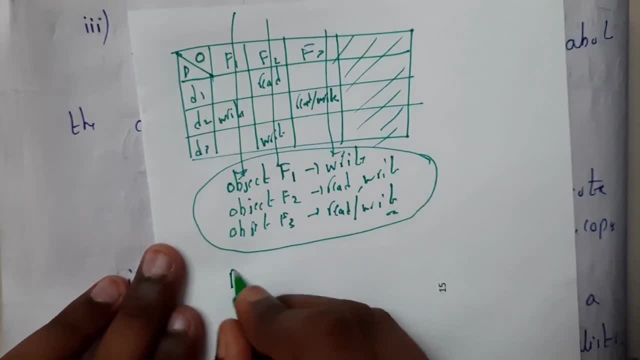 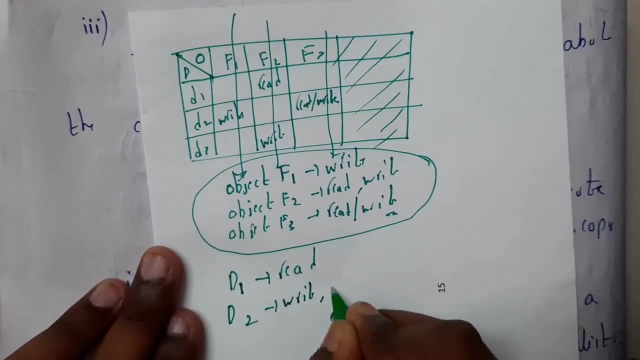 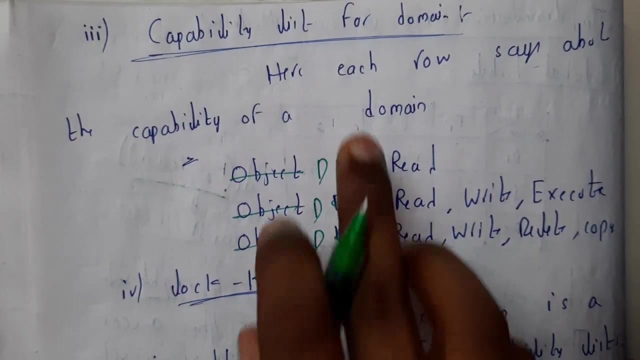 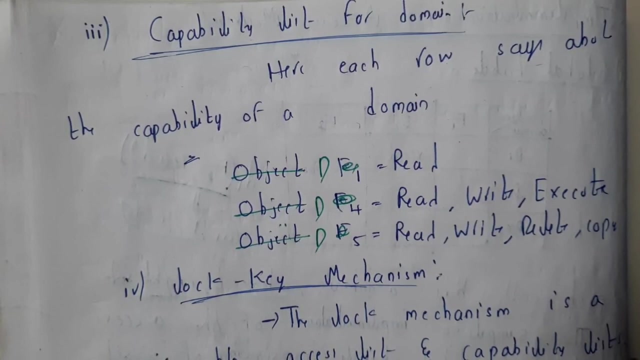 me to solve for this. so for domain domain one it will be read, for the main two it will be right or read or right, whereas domain b3 it will be right. so in this way we can do for capability list guys. so I hope everyone got a small idea on this capability list for domains. so there is a small other concept which 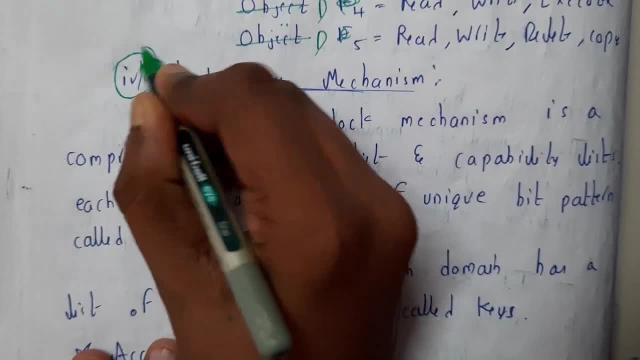 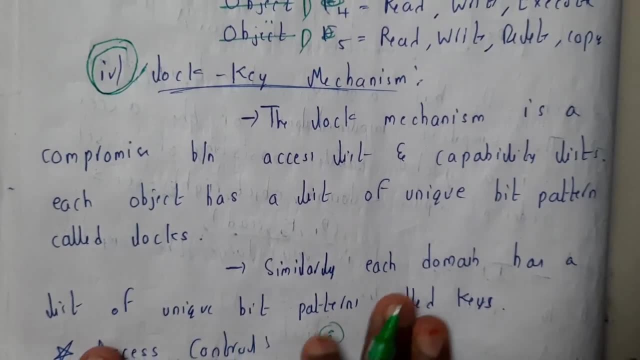 is lock key mechanism. guys, this i was not able to understand. i've seen many tutorials and i read from a book, but i didn't understand the main concept of it, so please go through the theory. i'll be just reading it out for you. so the lock mechanism is a compromise between the access list and 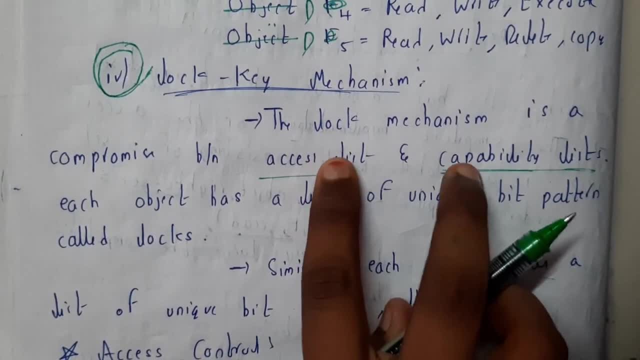 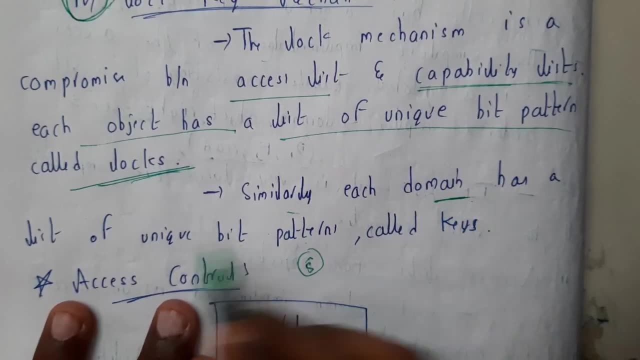 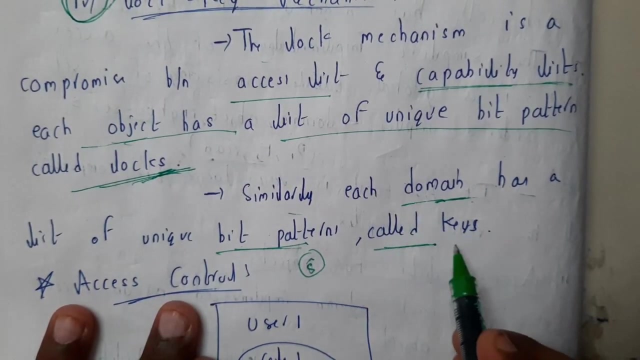 capability list. so it is a combination or it is a. it is in relation with these two, and each object has a list of unique bit pattern- locks- and similarly, each domain has a unique bit pattern that is called as key. so here we'll be giving: for objects we'll be having locks, and for domains we'll 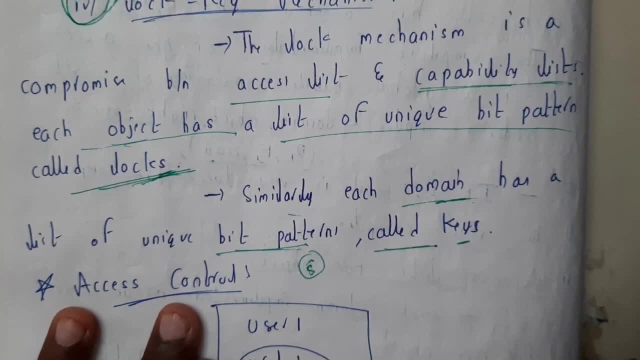 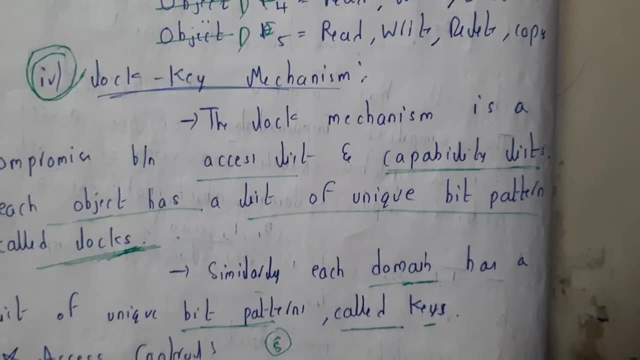 be having keys, but what is the use of it? i didn't get anywhere, so i hope everyone got a small idea on implementation of access matrix. so in the next tutorial we'll be going through access control, thank you. thanks for watching you.